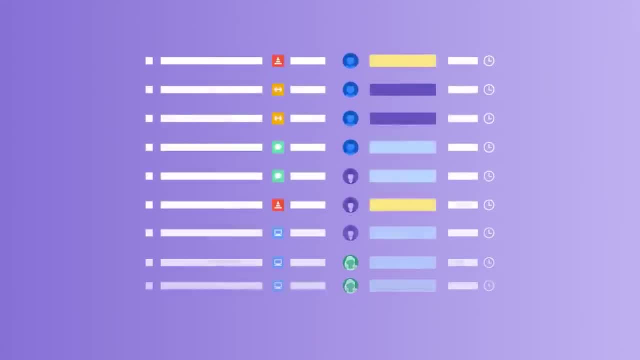 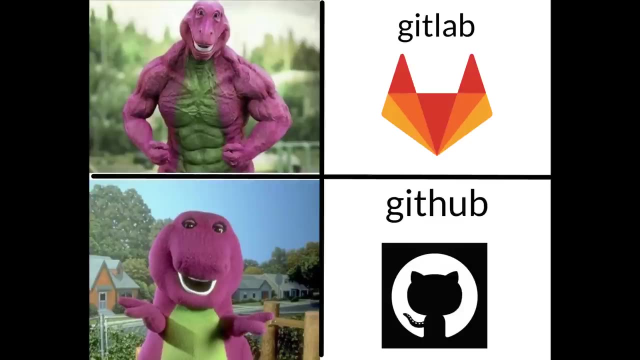 and it's hosted on a project management software. Sometimes it can be Atlassian Suite, so that's Jira, Confluence and Bitbucket, or it could be on GitHub or GitLab. Now that we're done- planning what we're going to do, estimating what we're going to do- 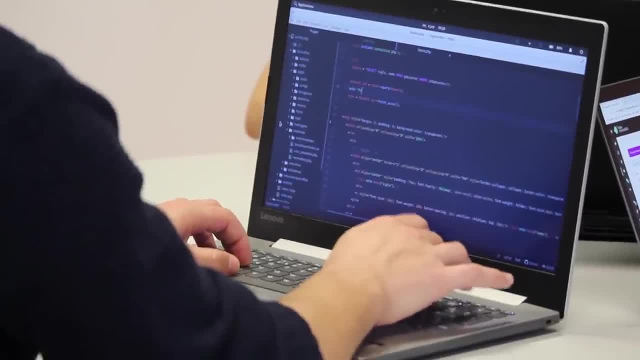 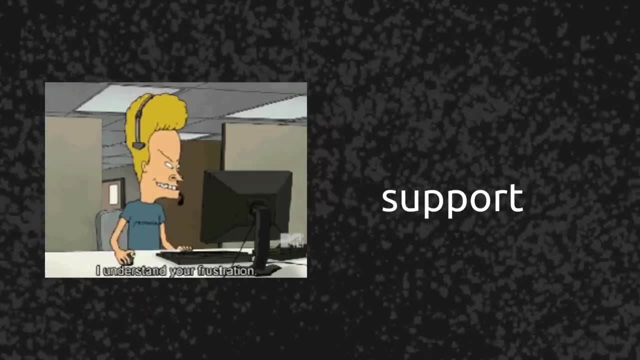 we finally get into the good stuff which is development, And as an engineer, you're probably going to get a few of the following tickets. So it's going to be a bug from customer support, maybe a new feature, an internal tooling And, if you're lucky and your company's, very nice. 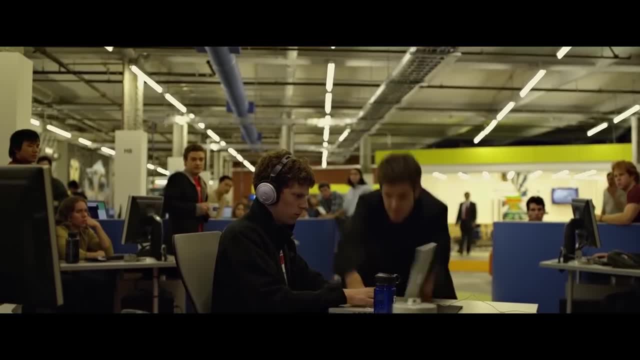 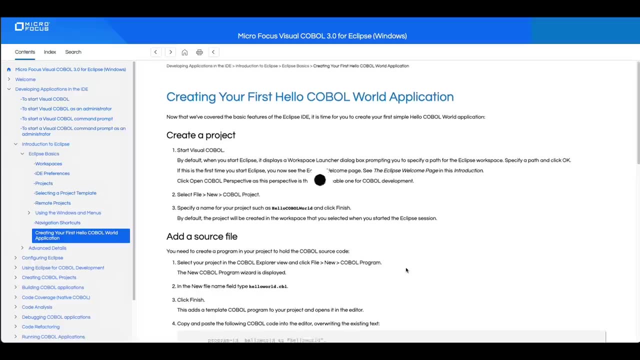 you'll get to refactor some tech debt. Now, while you're in development, you're actually going to spend a lot of time researching before you even code. So that means reading up on the documentation in the ticket, sifting through the code, Or, if you're 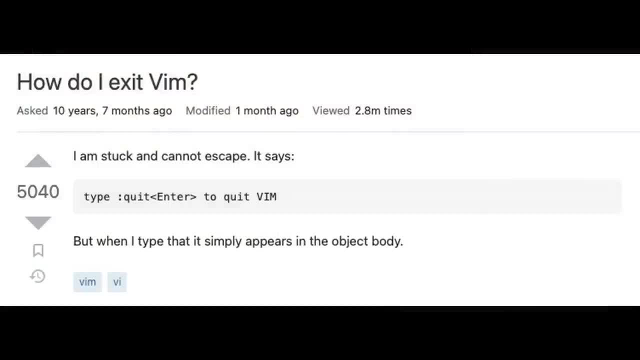 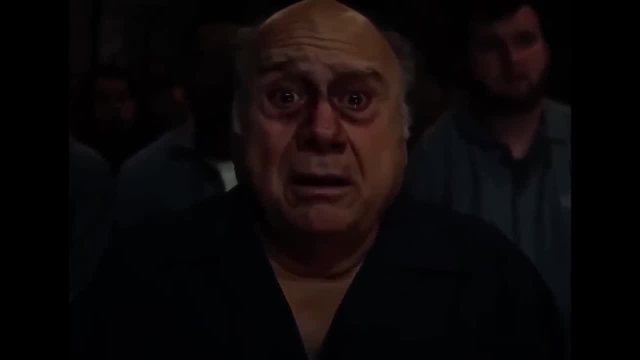 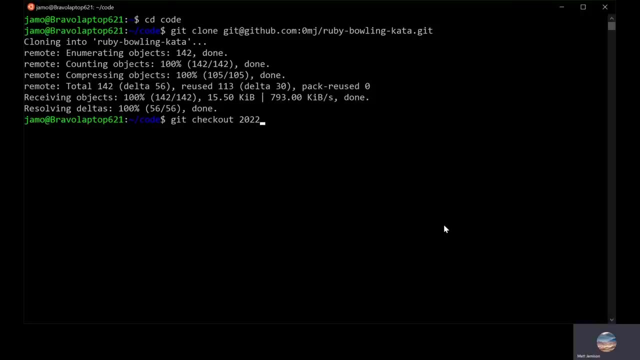 really new to the industry and this happened to me a lot in the beginning. you're going to spend a lot of time getting your environment up. Now that your environment's up, you understand the problem. you have a working solution in your head. you want to go and get check out a new branch and start. 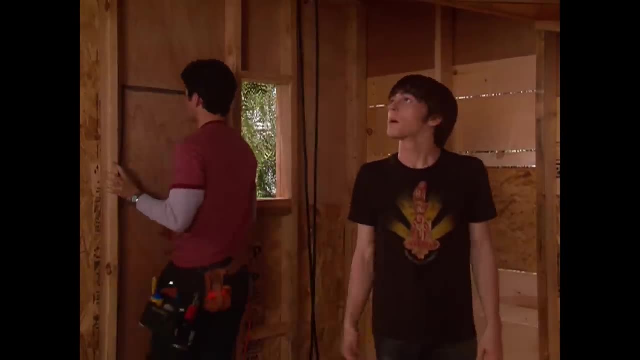 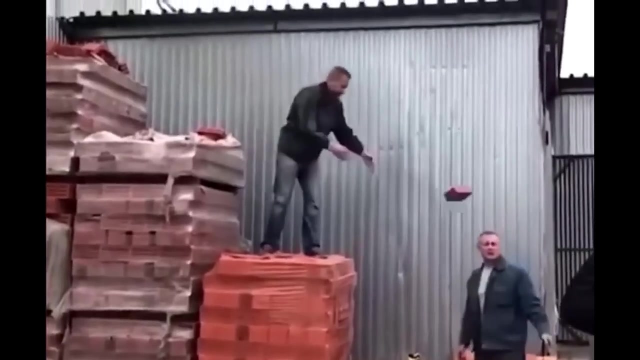 coding. So sometimes when you're coding it's very natural to be stuck or blocked by something that you don't really understand. And if you have a really good team culture, you can reach out to your teammates and they can hop on a call with you or come to your desk and you guys can work. 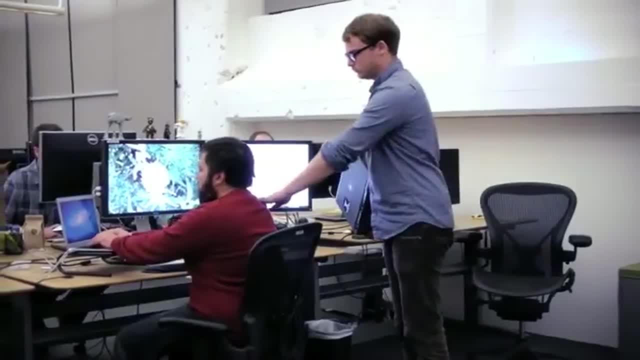 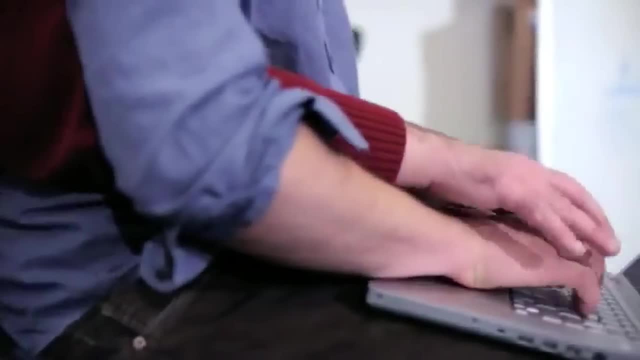 together. This is called pair programming, and it's very, very easy to understand and it's very, very popular in the industry because it's a really good way to build teamwork and actually learn a lot from your seniors and share knowledge. It's a fantastic practice and it's one of the ways 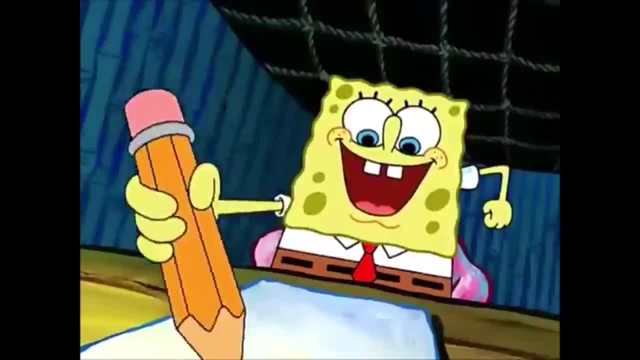 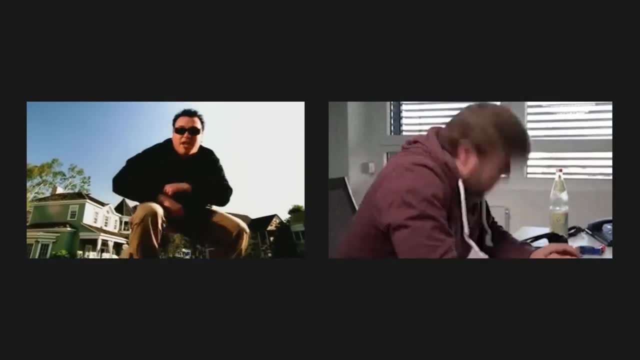 I've grown the most as a developer. So you fix the bug or you've built the feature, you've written your tests. you can now push your code and get it reviewed. Comments might start rolling in from other engineers or tech leads, And these are mostly about things like naming conventions. the 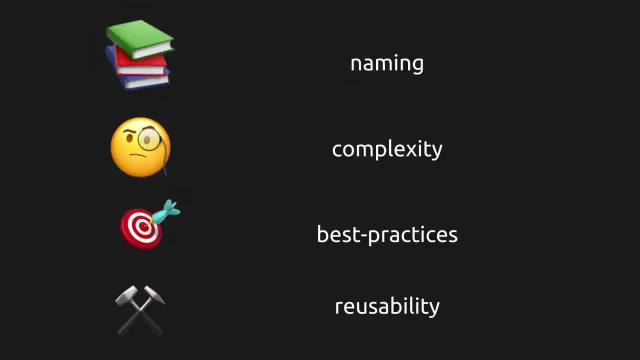 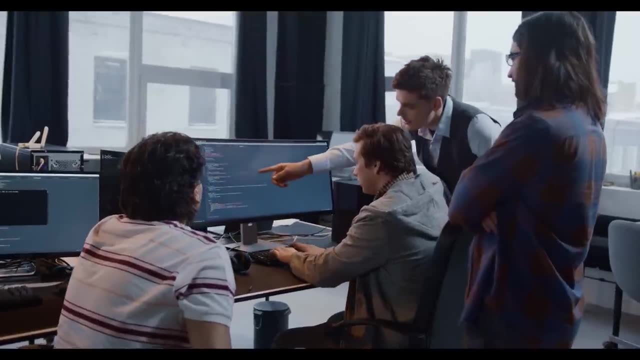 complexity of the code you've written, whether or not you're using best practices, whether or not you're using a code that's actually in the code And you can actually use it from somewhere else in the repo Once code review is done or while code review is happening. a member of your quality. 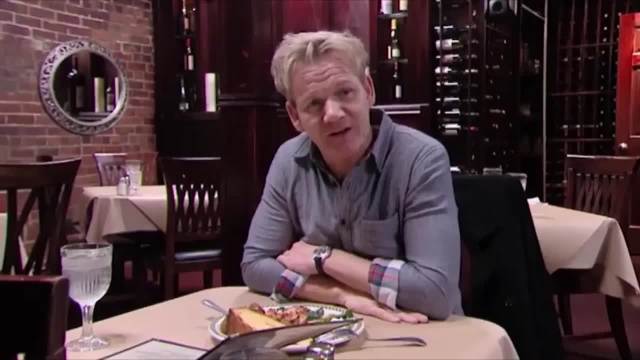 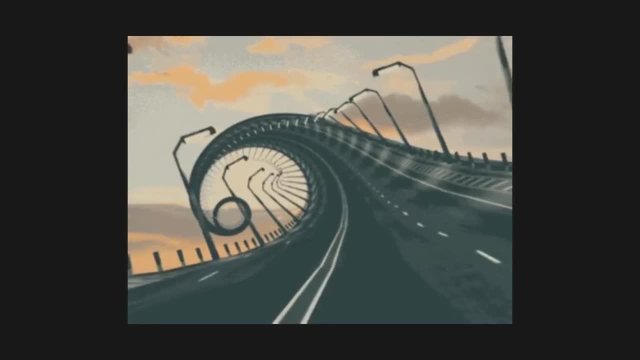 assurance team will pick up your ticket and test that feature. It's at this stage. if you have any bugs, you're going to have to go and fix it and get it code reviewed again, restarting the whole process. So for new developers, I highly recommend test out the QA tests yourself and make sure that.